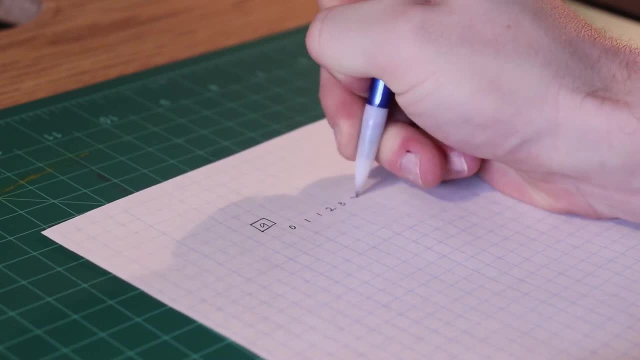 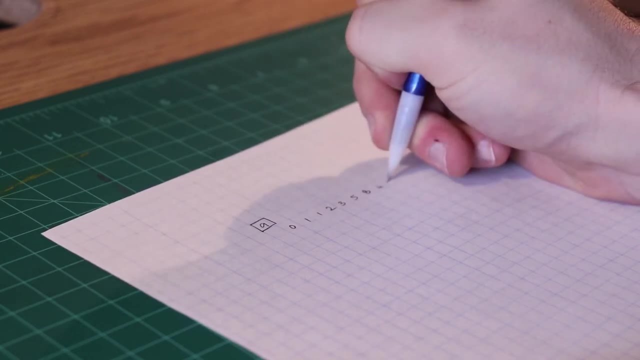 concept like the Fibonacci sequence, you already start to get a little hint that math can be applied in a visual sense, in ways that make sense for a lot of people, Which I think is important, because math is seen as really inaccessible for a lot of people. For me, I've been manipulating. 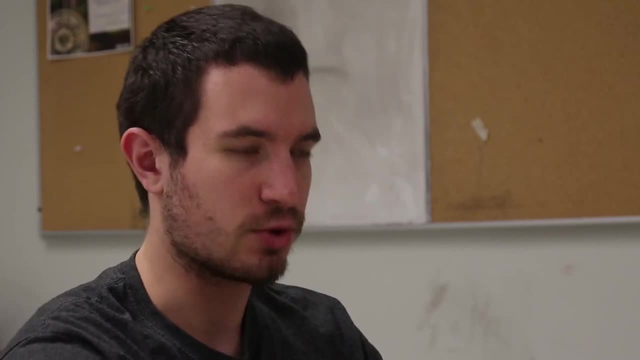 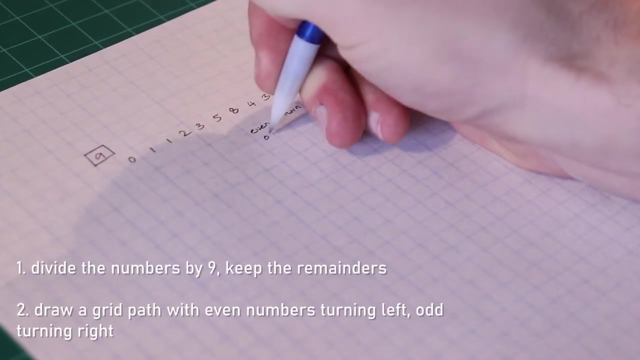 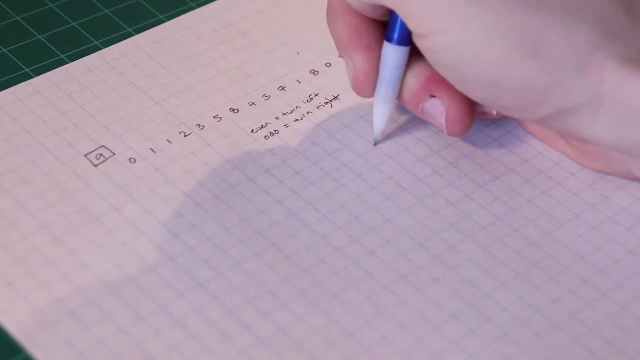 the Fibonacci sequence for a few years using a couple of rules, The rules that I've sort of set for myself that I feel are very fundamental. So I get these different sequences of numbers that are sort of derived from the Fibonacci sequence And after manipulating those, I try to figure out different ways to express those numbers. 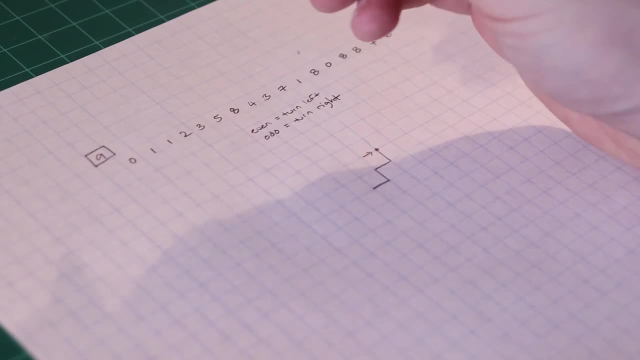 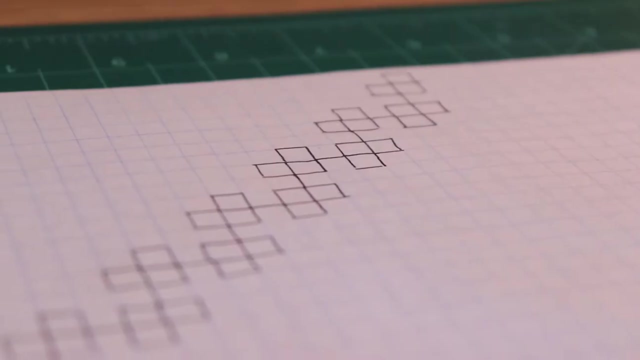 visually Set up some more rules for myself. So like, if I have this sequence of numbers, I draw a line for this number and it goes in this direction. If it's an odd number or an even number, Like I have a design set that's based on graph paper. 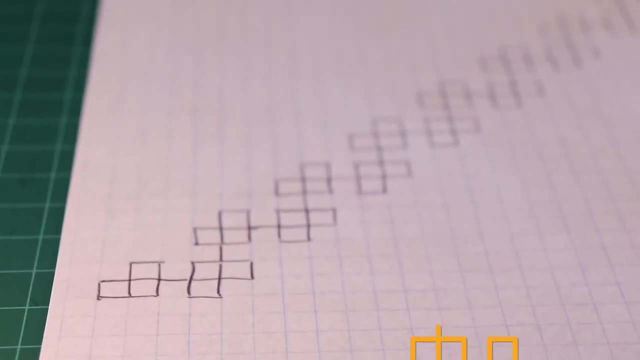 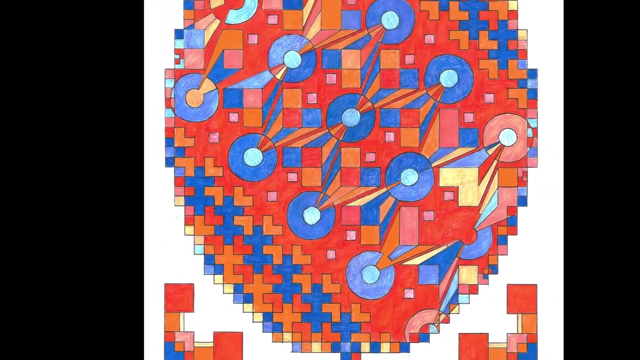 It might not look like much once the sequence is done, But you do have a shape that could be used for. it might be a good floor tile design. It might be good for something else, You don't know. Take all of the digits possible in the sequence and set them up in a circle, And then I draw lines. 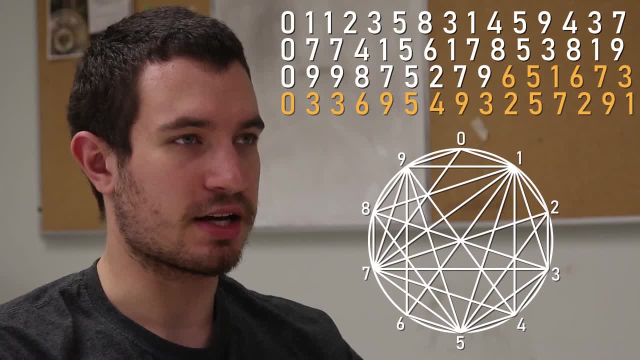 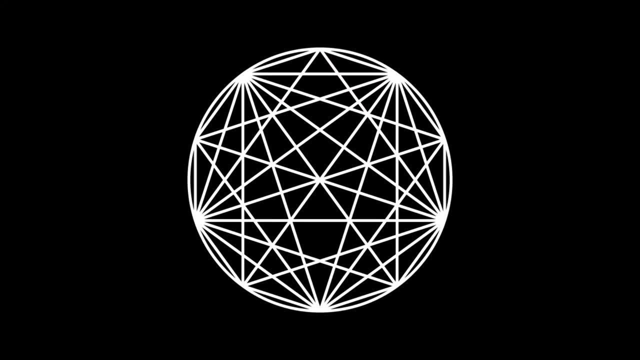 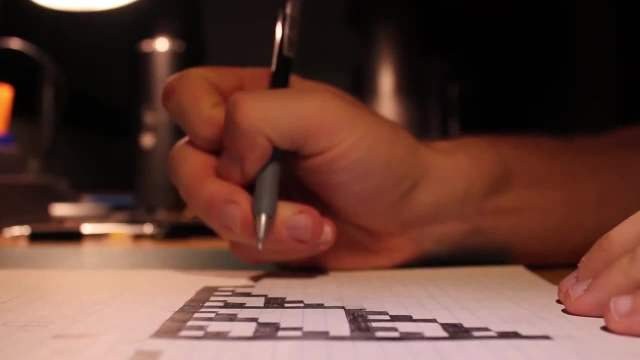 between them, based on how they are arranged in the sequence. And I get these, just these really interesting shapes, which maybe aren't really seen, as you know, fully fledged designs in themselves, But they could be basic, Like building blocks for something bigger. You apply a couple of rules that you set for. 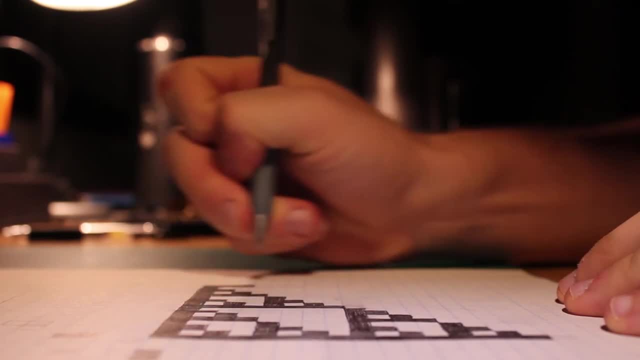 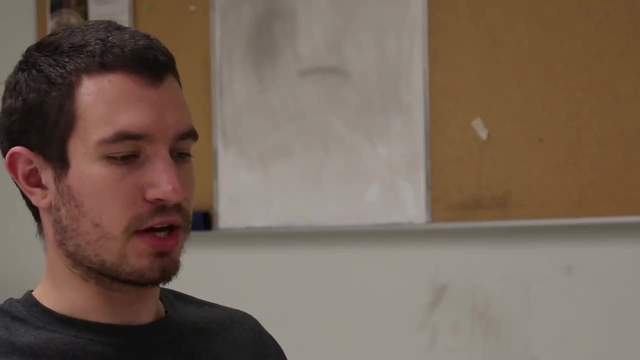 yourself and then you just see where the result takes you And it produces shapes in the end, or lines even, And then you use those lines and shapes and maybe you add more rules, so maybe you get more intricate shapes, more intricate lines and you keep producing these kind of 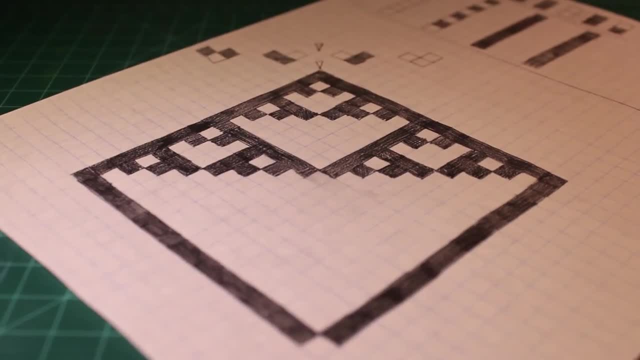 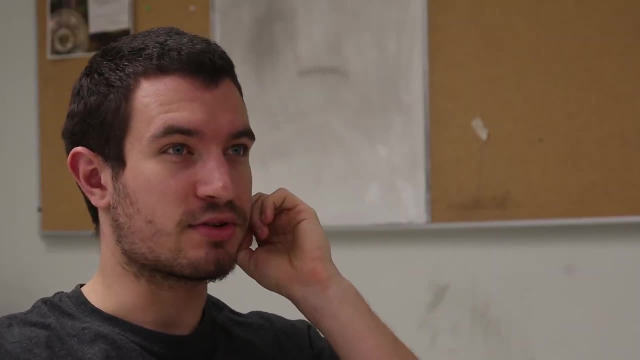 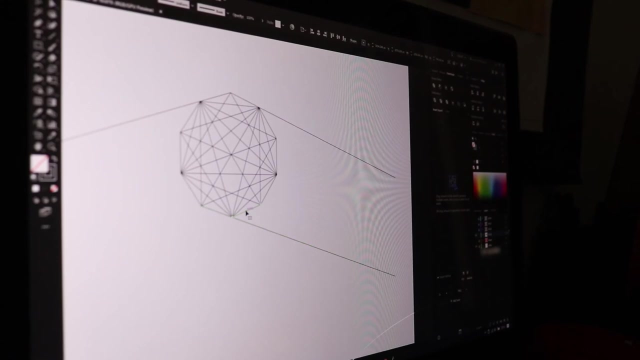 building blocks that you can use for other designs. So then you have this whole concept of like. Okay, well, how? how much of this art that you make via instructions that you assign for its creation process, how much of it like? there's a whole like individuality, like identity thing along with it?